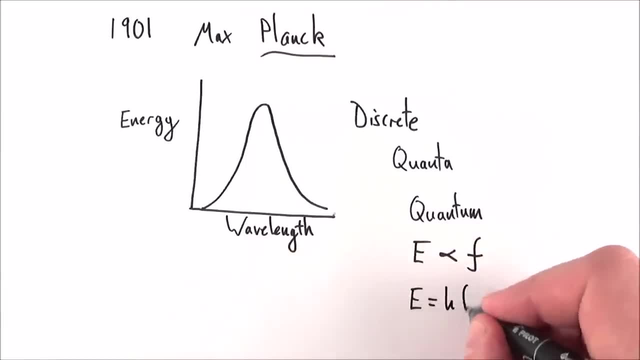 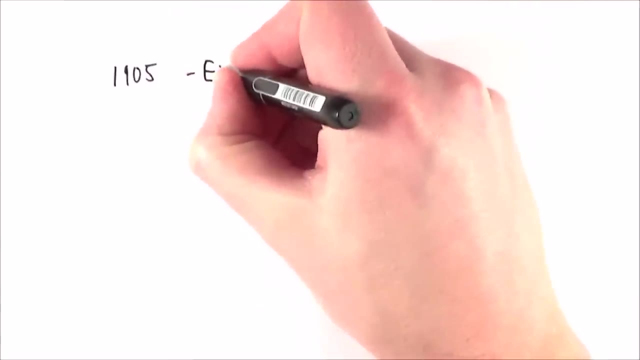 which is what is called Planck's constant. so e is equal to hf, but that wasn't exactly the photon. okay, this is just saying there's a link between the energy emitted and the frequency of that emitted radiation. but it was four years later, in about 1905, that Einstein really sort of published. 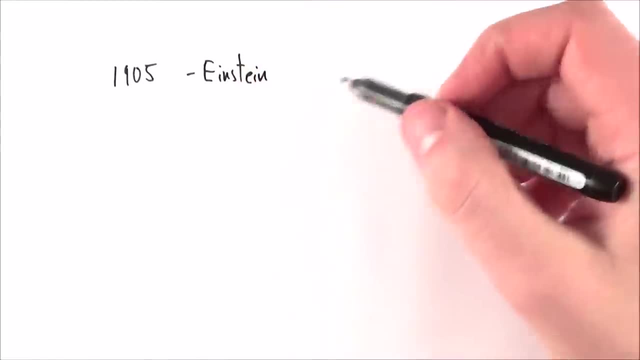 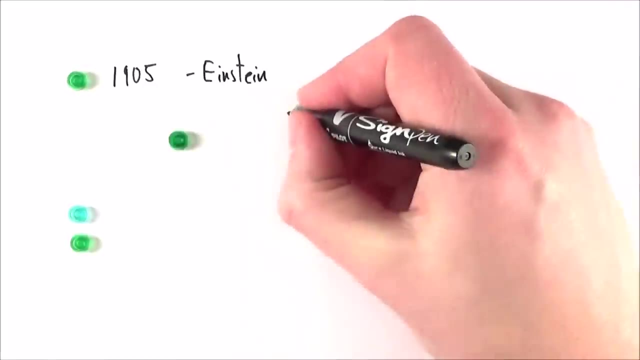 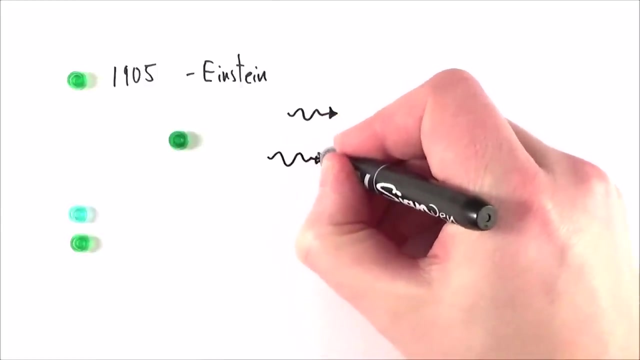 his work on the idea that energy isn't just emitted in a discrete packet of energy, but it actually continues, and this concentrated packet of energy has particle-like properties, sometimes given a symbol a bit like this, to show that it's a discrete little packet of energy, and this is what 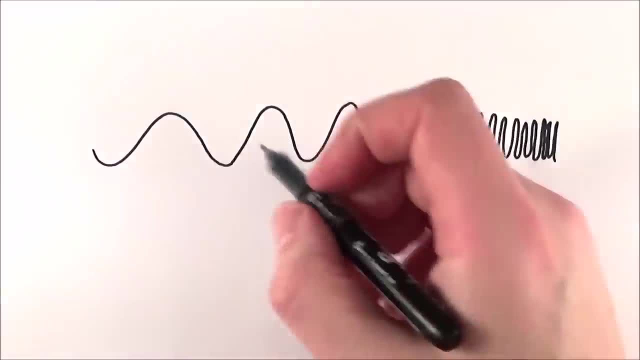 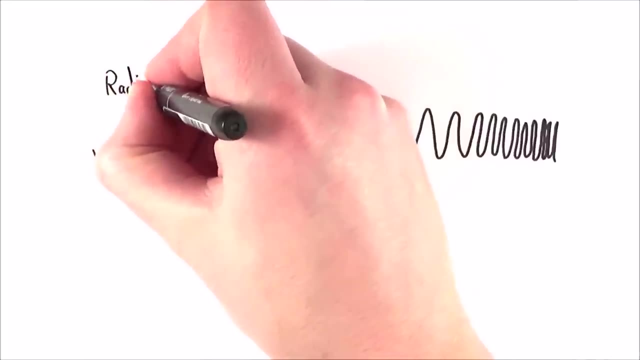 is called a photon. Here we have a rather badly drawn picture of the EM spectrum, which you've already had a few videos about, and what we find is that we have waves, as we think about them, going from radio waves at one end through to gamma at the other. So the idea that Einstein really came 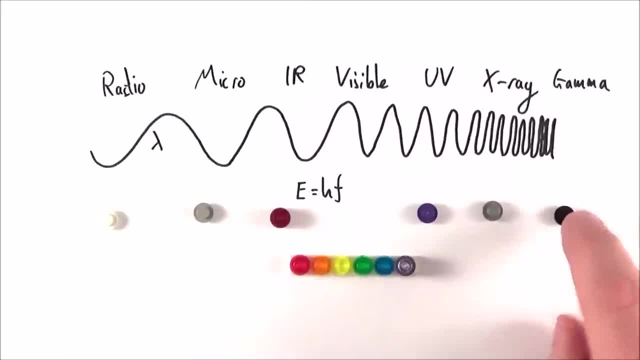 up with is that energy exists in these discrete packets of quanta and we maybe had the low energy photons at one end, moving through the higher and higher energies, the visible light going from red through to violet, then the ultraviolet, which is more energetic. there's more energy in an x-ray photon and finally the gamma ray photons are the most. 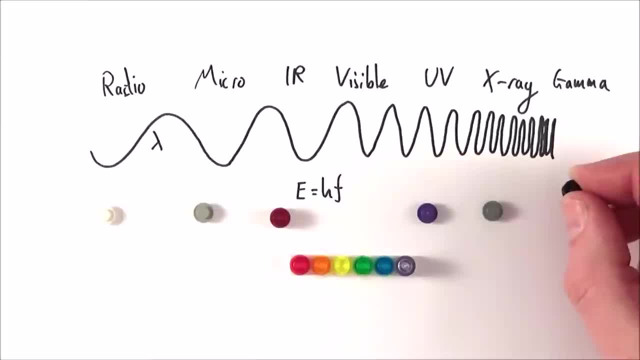 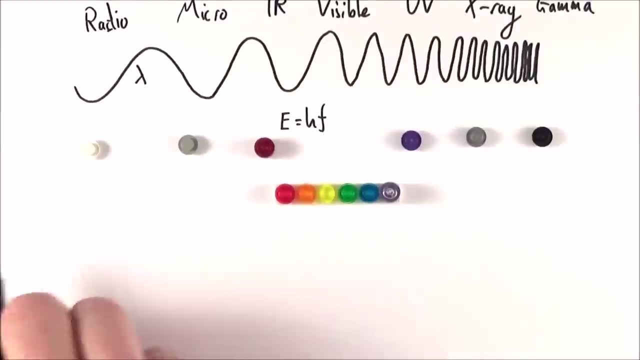 energetic of all, and that's because these have the highest frequency waves and therefore they may have the most highly energetic photons. So what else do we know about these photons? Well, you know, we know certain things. perhaps, if you have maybe three photons combining together, that does effectively give us the white light, for example, which is why would it have the white? 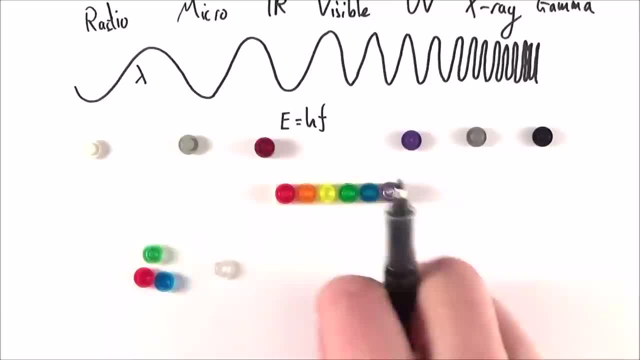 light in the spectrum down here. Also, the things about the photons that we need to know is that they are massless. okay, so they have no mass or their rest mass is equal to zero, and what that means is that they therefore travel at the speed of light, or, in actual fact, they can only travel. 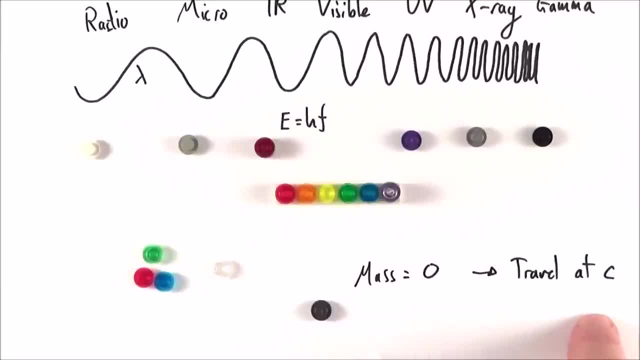 at the speed of light. Anything that has no mass only travels at the speed of light, for example, some of the exchange particles, in which case the photon is one of those, and anything which does that can never get to the speed of light. What else about it? Well, we already know that E is equal.